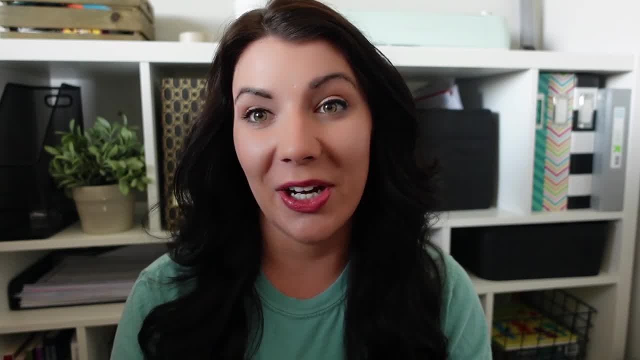 all things pre-k, so I won't be including those in this video. This video is part of a collaboration hosted by Shauna from Homegrown Homeschool and Devine from Calm in the Chaos. I have done a bunch of collabs with these wonderful ladies and I will link both of them in the description box. 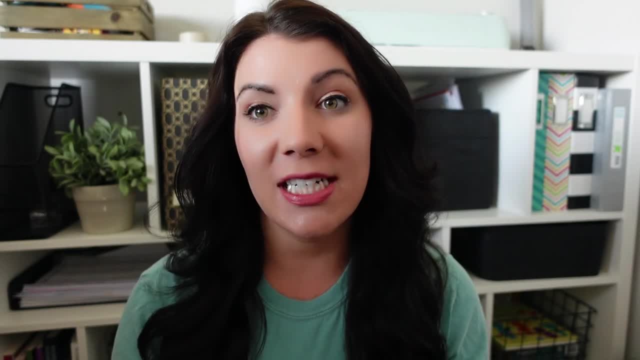 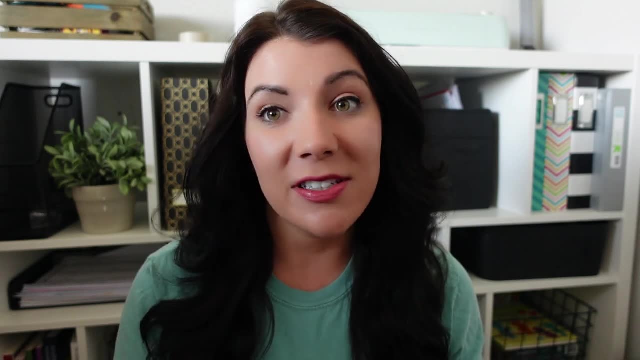 Their channels down below and the entire playlist. so if you're interested to see just a bunch of different language arts curriculum and approaches, you know, piece it together. do they use an all-in-one? you'll definitely want to check out the entire playlist down below. So, like I mentioned, my 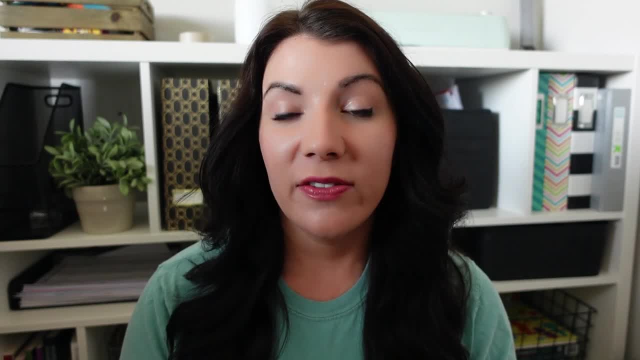 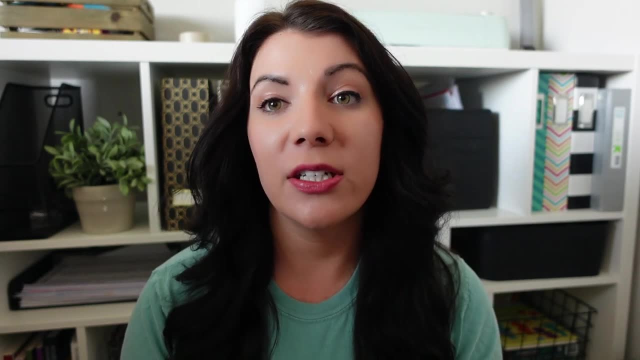 soon-to-be fifth grader and third grader. they do a lot of these subjects together. that that's not how it's always been. When we first started homeschooling and for the first couple years, we were using the good and the bad. We were using the good and the bad. We were using the good and. 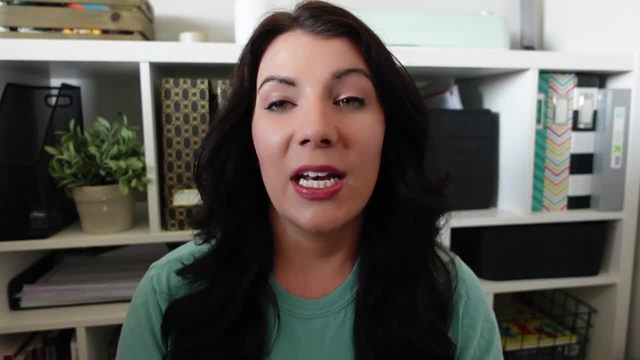 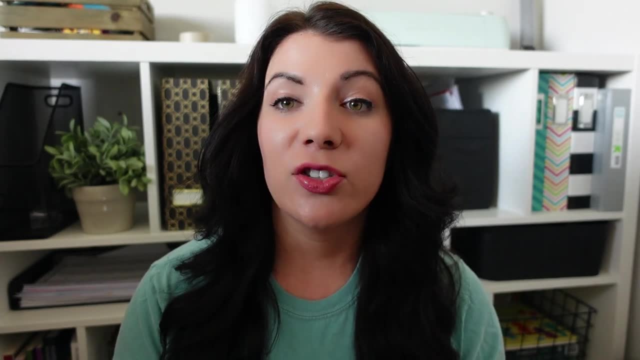 beautiful, It was easy, It was open and go, Everything was in there. but it just stopped working for us at the beginning of this current school year and so midway throughout the year we switched and we started really piecing together a lot of our language arts curriculum, and that is. 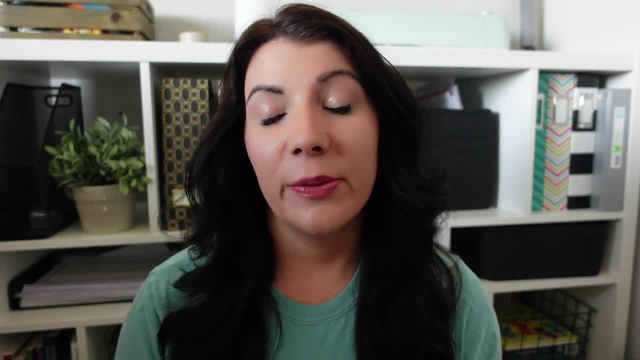 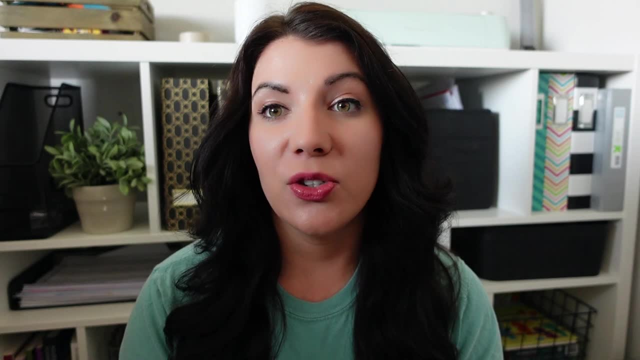 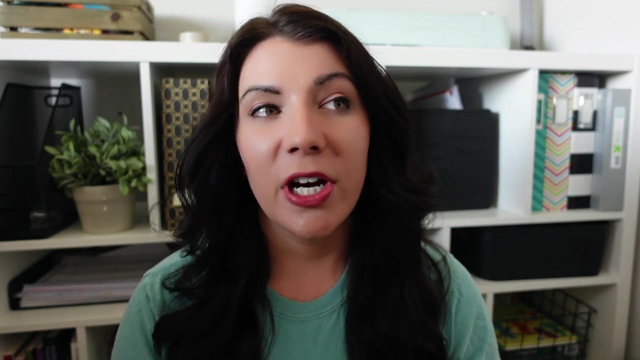 why my daughters do it together now is because a lot of the curriculum I found kind of spans over age ranges Because they are two grade levels apart. I do sometimes have you know, a little bit stricter of rules. My older daughter has to follow a little bit more lenient with my younger daughter, or we take a little 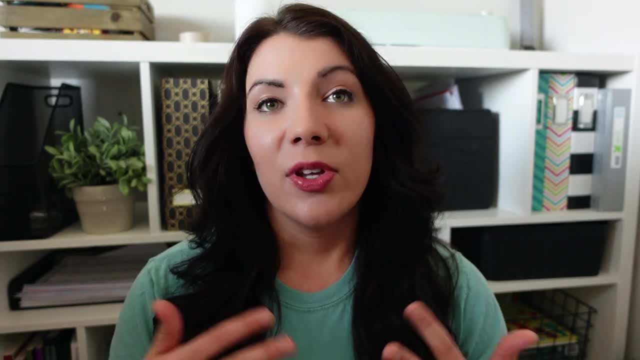 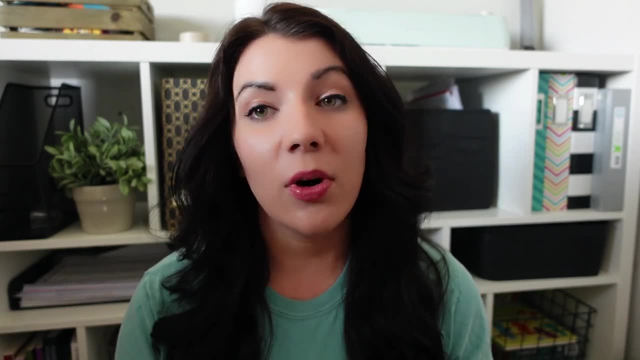 bit more time to complete things or, to be honest, you know, for reading a more challenging book, and my older daughter is the one who's like answering the discussion questions a little bit more, then we kind of just go that route. I don't want. I want to cater to both their ages, but 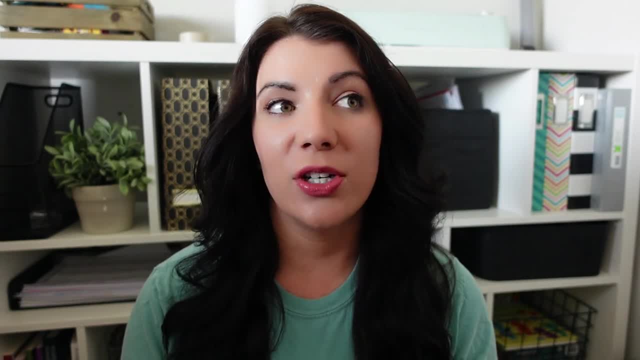 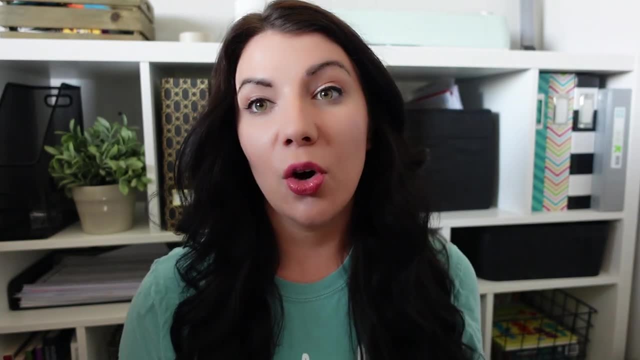 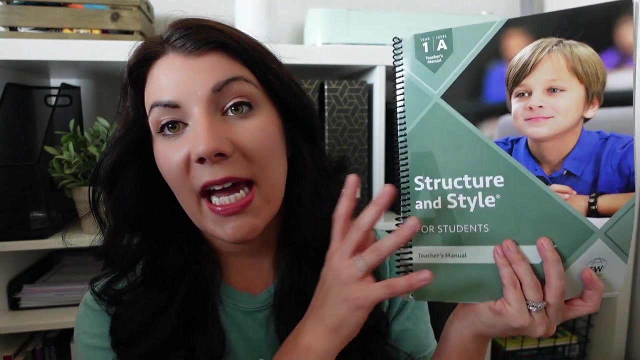 I don't want to hold anyone back and I also don't want to, you know, cause frustration either. So we're always adapting and that's how we make it work with the two different grade levels. So for writing, we are using IEW structure and style, year one, level A, and so this was something we 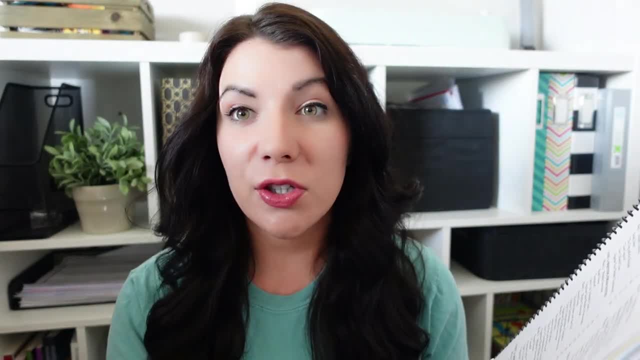 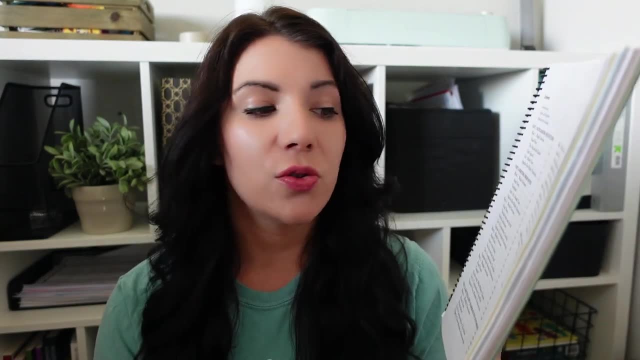 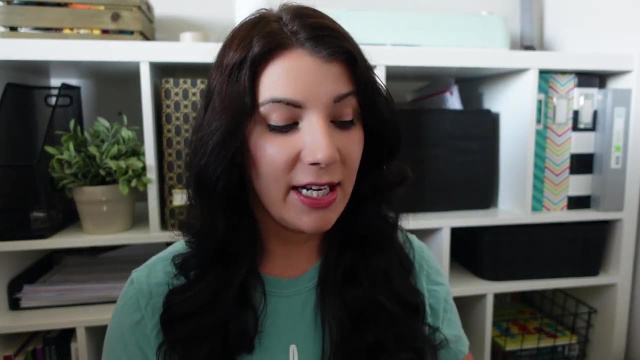 actually started this current year. We did the first three units, so we did units one, two and three and then we stopped, and so when we start this new school year, we'll be starting on unit four and completing units four, five, six and seven, and so we may end this early, before our school year. 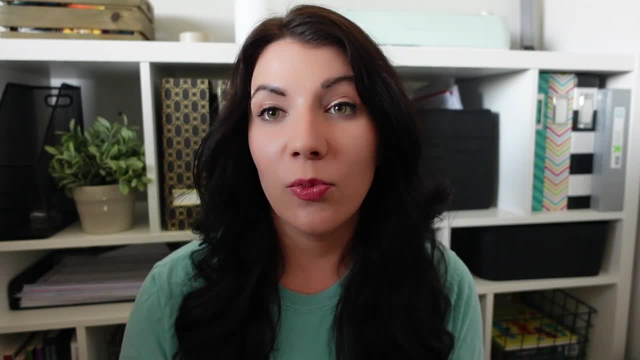 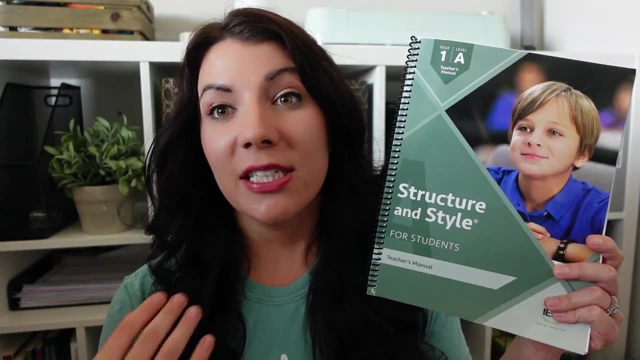 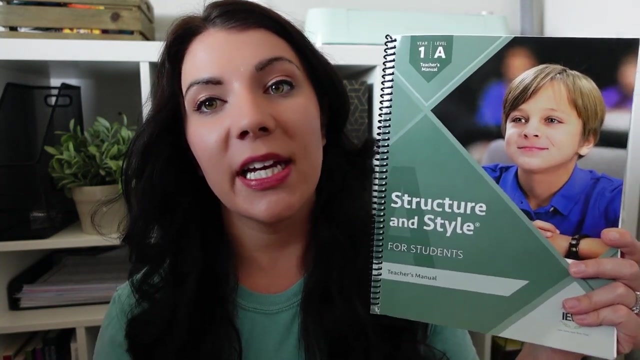 Our next school year ends and we'll either, just, depending on where we're at we'll, get the next level or work on something else. But this is for grades three to five, and so, even though we started it this current year, my current second grader has been able to keep up, but, like I said, I'm not as 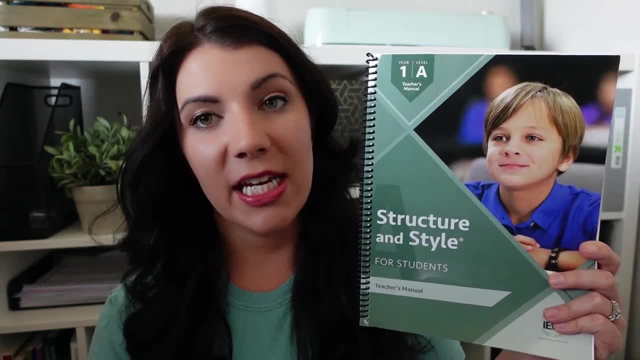 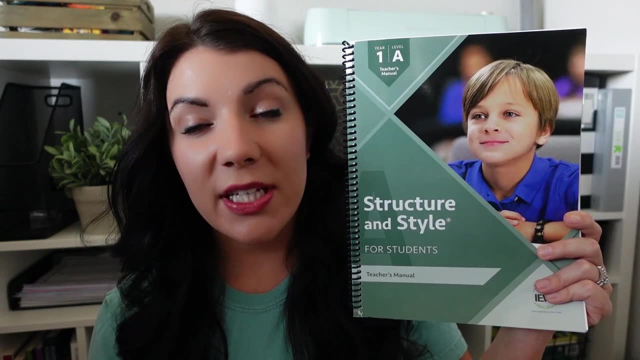 strict with her because she is a lot younger taking this course. So we kind of just adapt it, I think, for like one week of lessons. we normally spend two weeks doing it, And that's one, so they don't get frustrated with it, and two: we only homeschool three days a week. 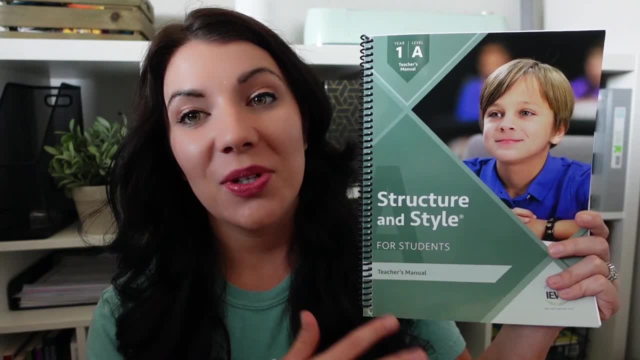 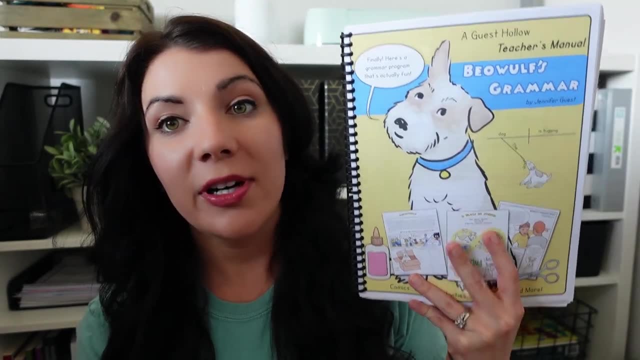 and so we cram a lot of stuff in those three days. So this spreading it out over the two weeks really does help. We've also been using from Guest Hollow, Beowulf grammar. This was also something we started this current year. We did the first- I don't know- like the first semester, I guess I think it's like. 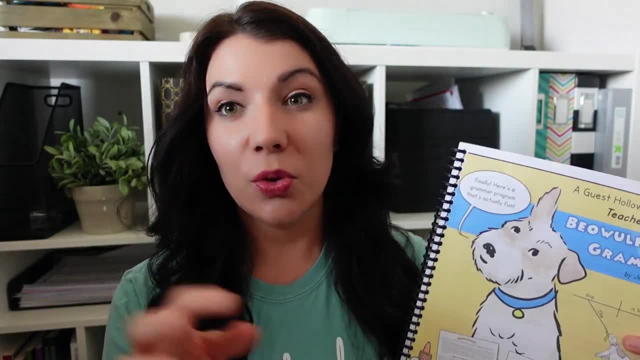 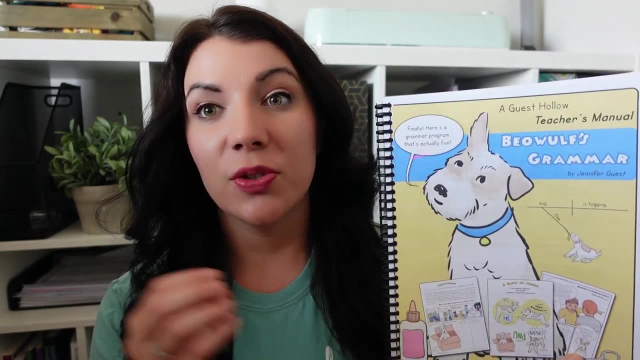 the first 10 weeks and then we have, I think, two more semesters or three more semesters. So again, this will take us into our next school year. This ranges from grades two to six. So same thing. I kind of just go a little bit more in depth with my older daughter and keep it pretty, you know to. 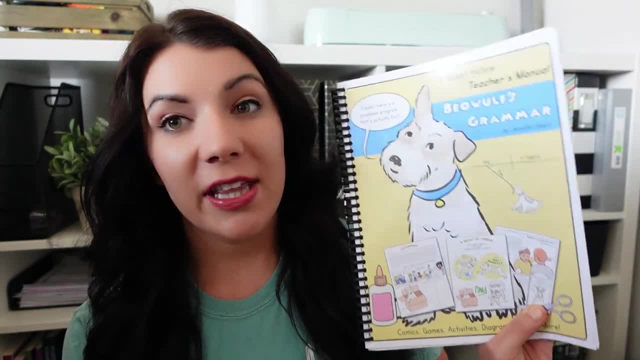 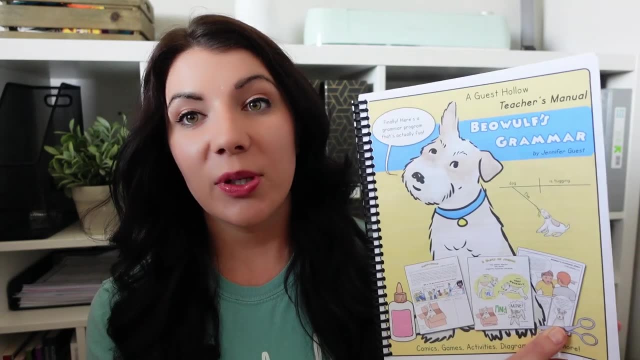 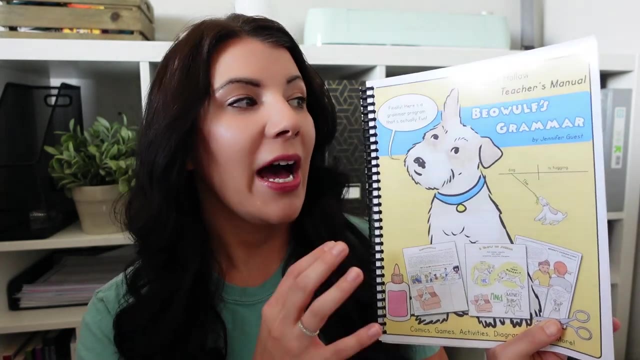 the point with my younger daughter. After this we will be moving into Fix It grammar. So we did try Fix It grammar and we really liked it. My kids really liked it. I just felt like they needed a better base level before that type of curriculum is used. So I know for sure after we get into the 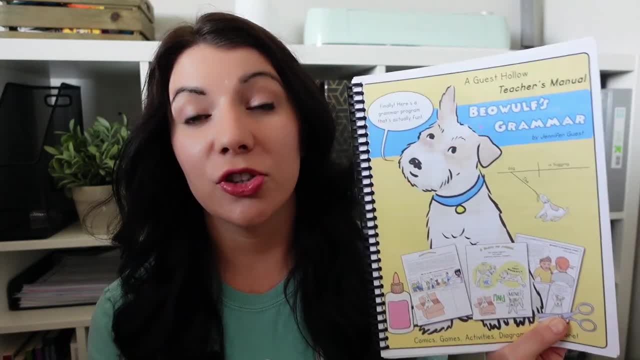 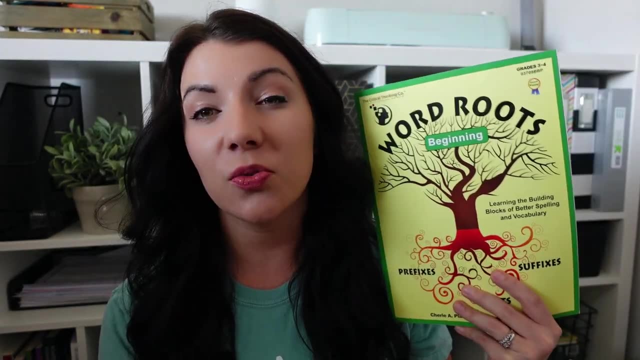 all of this that they're going to be great for Fix It grammar and that will transition into For spelling and vocabulary. we have been using word roots. This is the beginner level, So this is really getting them to understand just the concept of a root word, of a prefix, of a suffix. 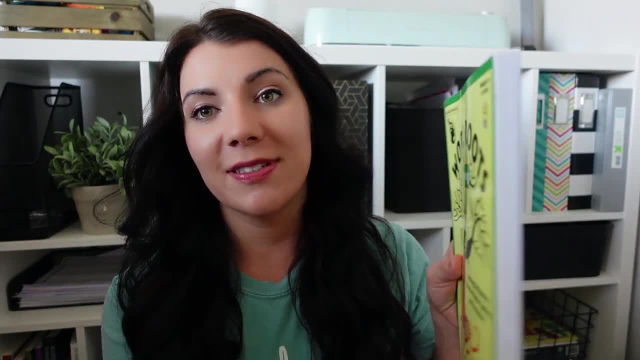 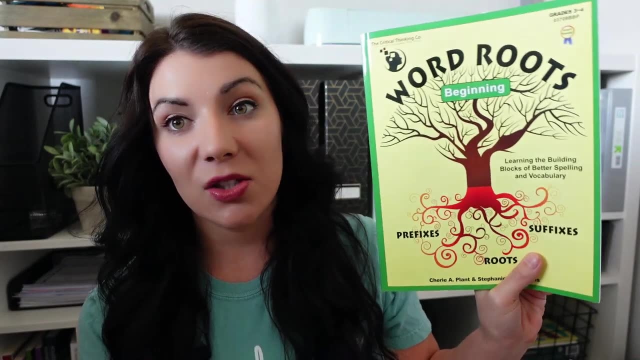 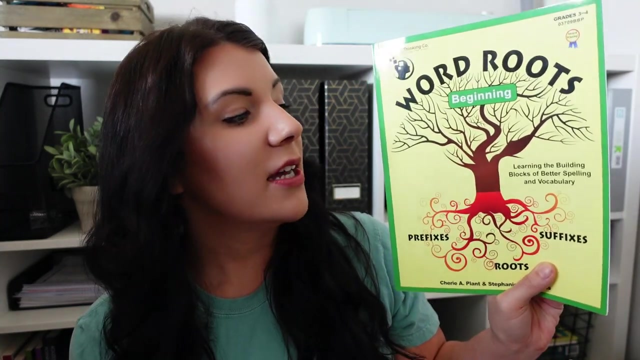 And so this is a one of the smallest word roots levels, and this is for grades three to four, And so we've started working through this, and, again, this will take us into our next school year. Once we complete this, then we will move on to level one, Something I've been doing with these. 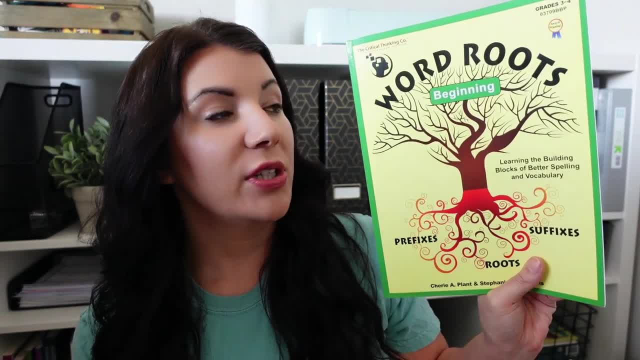 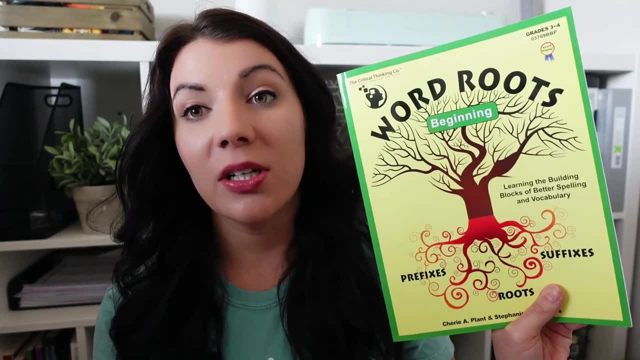 words for my older daughter is. I have been treating the words that she's learning as spelling words and kind of having her test on those. So that's kind of the only adaptation between my older daughter and my middle daughter is my older daughter gets tested on the spelling of these. 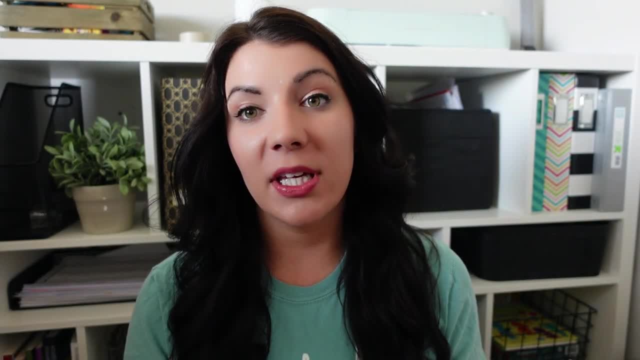 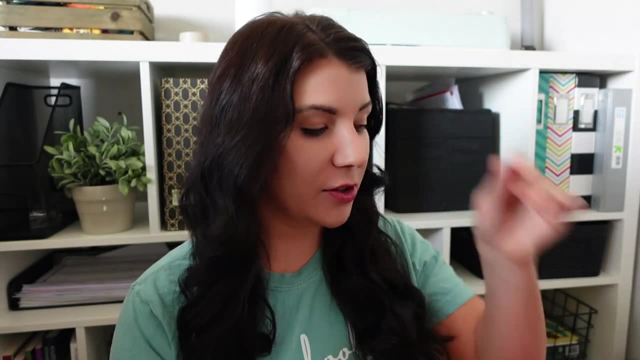 words. Both my daughters will continue doing handwriting this upcoming year. They both are learning cursive. My current second year is going to be cursive, So I'm going to be doing cursive. She has started cursive. She is doing the first book from Handwriting. Without Tears- I don't. 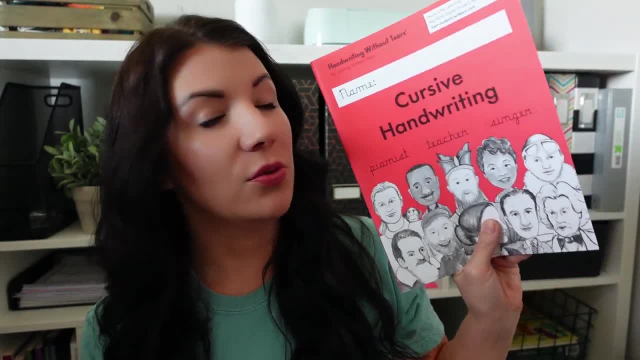 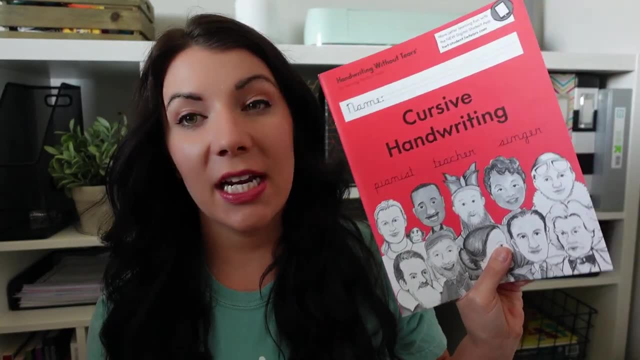 remember what it's called, But she's about to complete that, and so then she'll move into this one. This is our first time using Handwriting Without Tears. The level before this is what she's working on, and I do like it. It's a little bit different. The only thing that I've noticed. 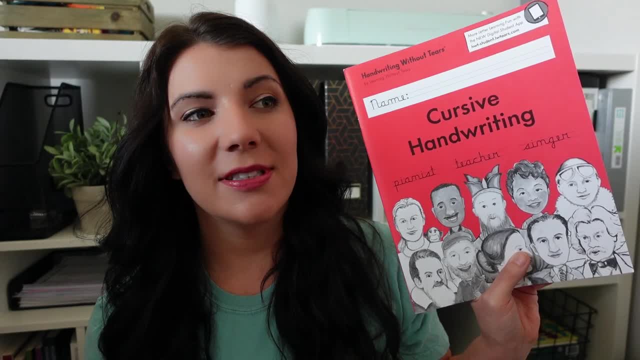 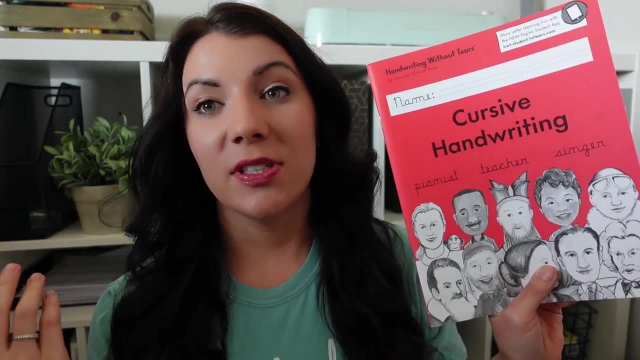 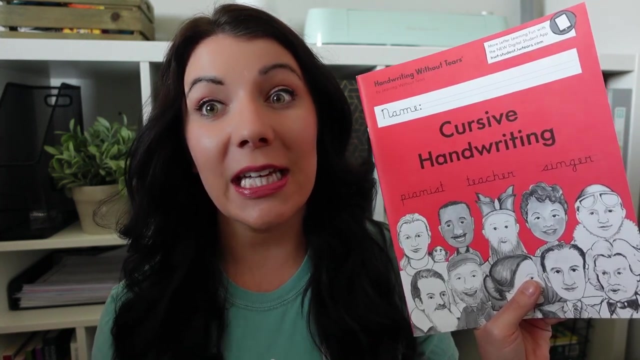 is. I think it's letter Q or Z, I can't remember. It's done differently in or it's Q. It's letter Q. Older daughter has been using the Good and the Beautiful handwriting and it just happened they were both doing a handwriting cursive page with Q's and their Q's looked completely different and 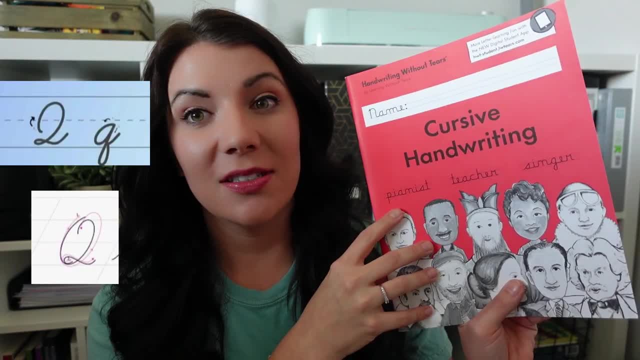 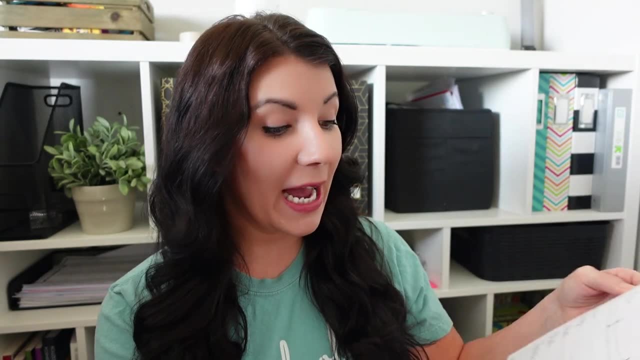 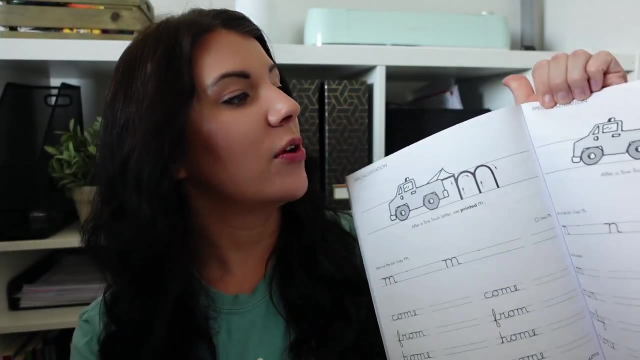 I was so confused, And so the way that this teaches Q's is not what I'm used to, or traditional, as well as just the way that this cursive is kind of laid out. I think it's good for younger students learning cursive, but I mean, this is more than halfway through this book and it's still just. 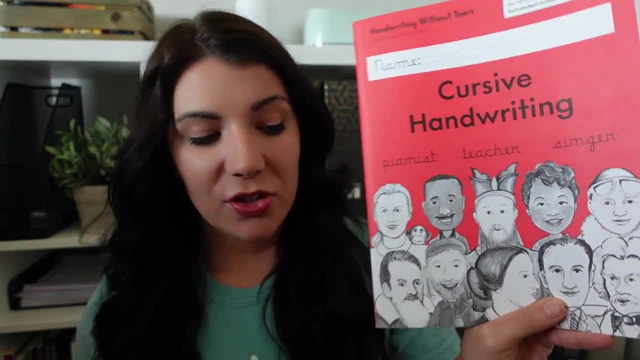 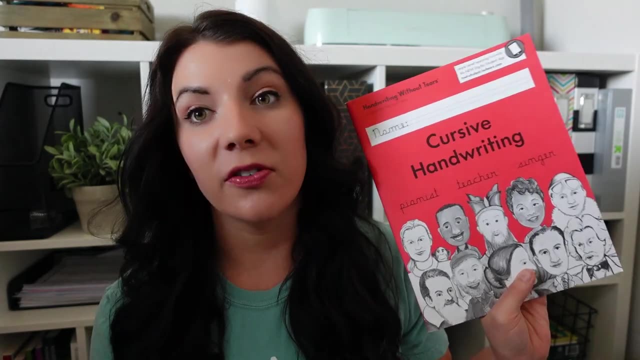 like a mix of print, I guess in cursive. So I don't know if I'm going to end up changing this either back to the Good and the Beautiful, because we've just used that and that works, or looking for something different. We will see. And then for my older daughter- she's already done a few years of. 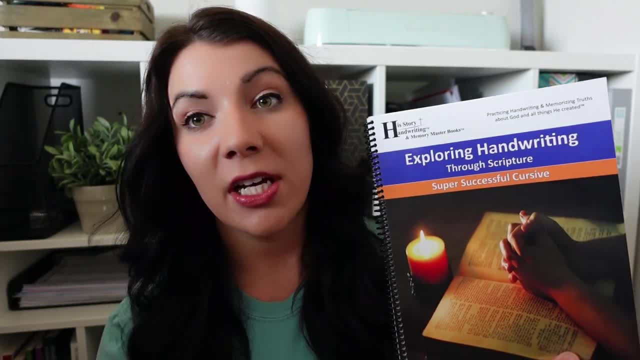 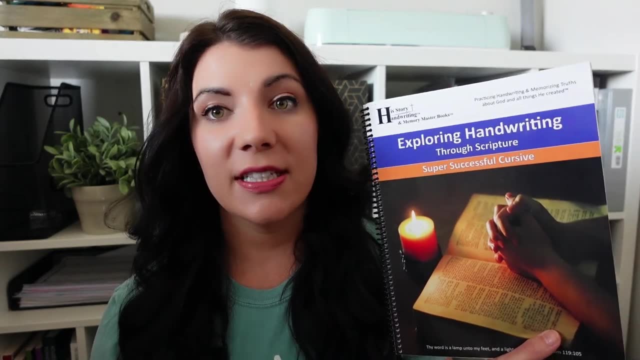 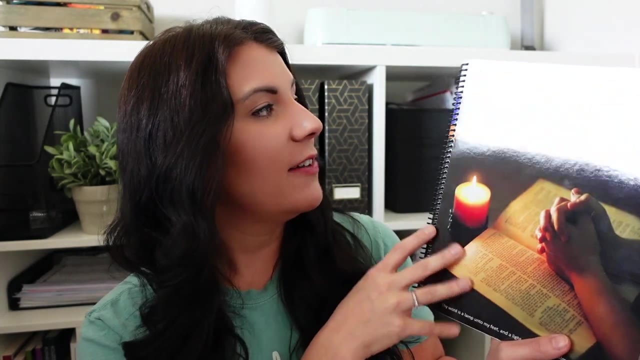 cursive and she has the basics down. She knows how to write all the letters. She really just needs to work on continuing to practice. make really like formulating her own handwriting style. No more you know, re-read something and write it, And so I found this: His Story Handwriting. 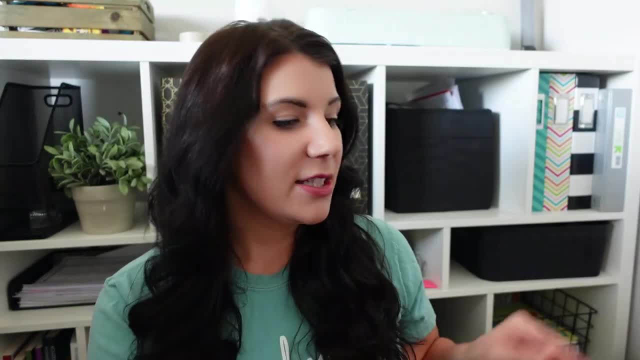 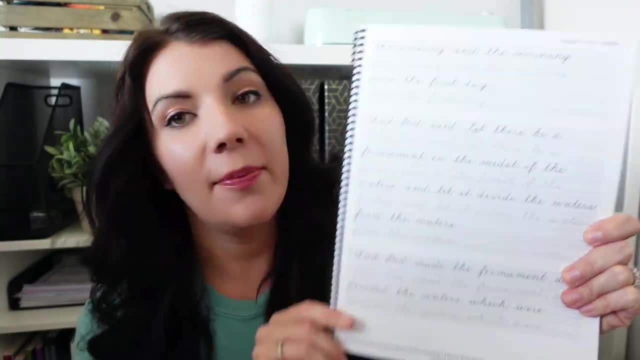 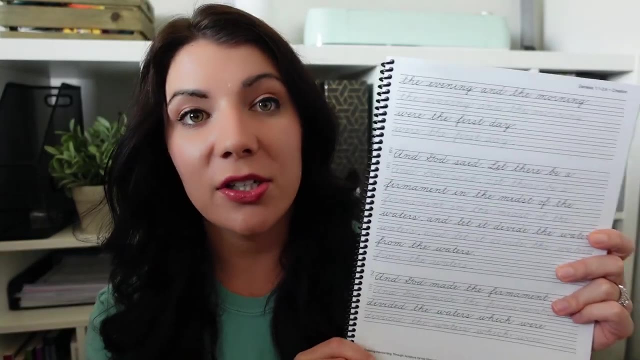 exploring handwriting through scripture, And so basically, she's just reading verses and scripture and she's just rewriting them, copying them. It's a lot smaller and closer together. This will also help her continue to develop being able to read cursive. That's something that is a little bit more important to me. I don't want them to be. I don't think that. 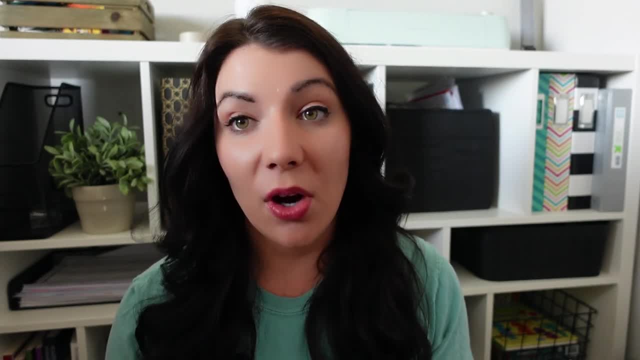 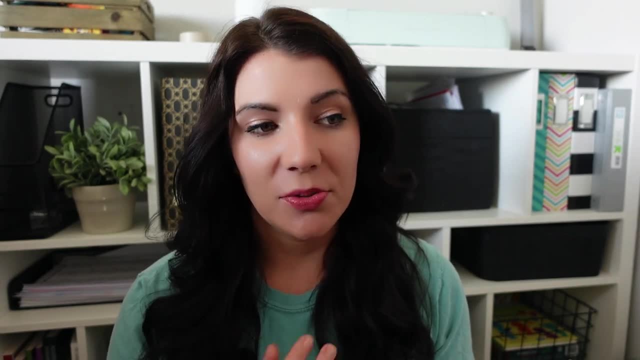 they're going to be writing papers in cursive. I think they're going to use it to develop their own handwriting, But I really want them to be able to read cursive and older cursive. So what's really funny is my grandmother, so their great grandmother, she. I get her groceries for her every. 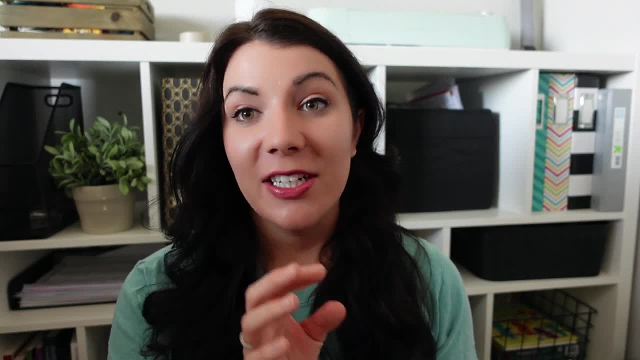 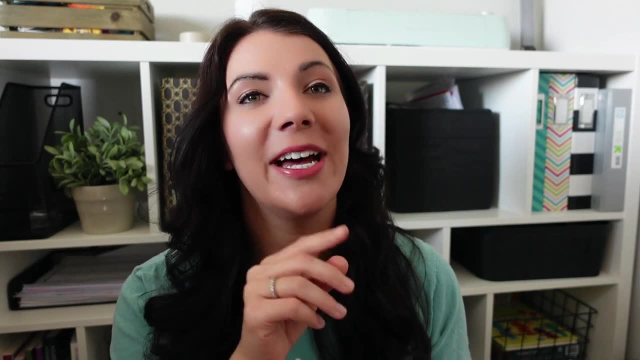 week and she writes a list in cursive and she has like very difficult cursive to read because it is just well. first of all she writes in like a light purple pen, so that always makes it really fun, But it's like super close together. 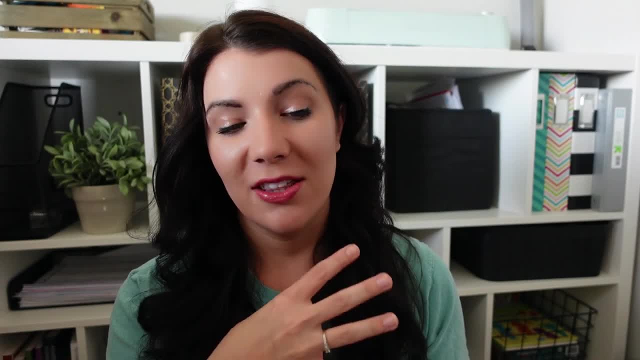 So what I'm going to do is I'm going to take a little bit of time and I'm going to go through it. So we've been just practicing. I'm like, tell me what's on the list, and they're kind of you know. 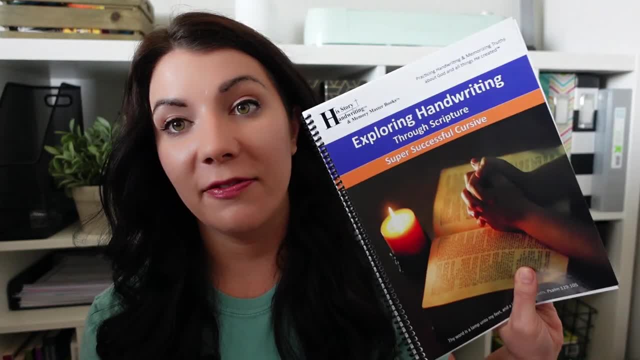 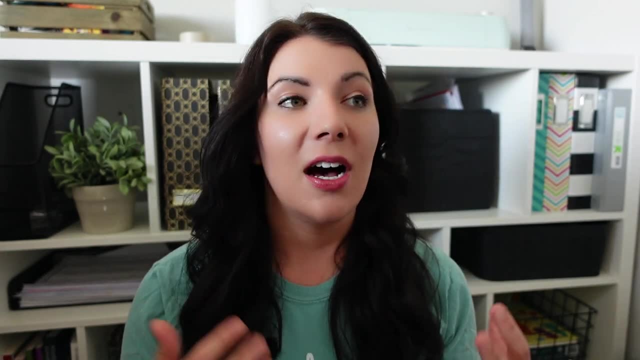 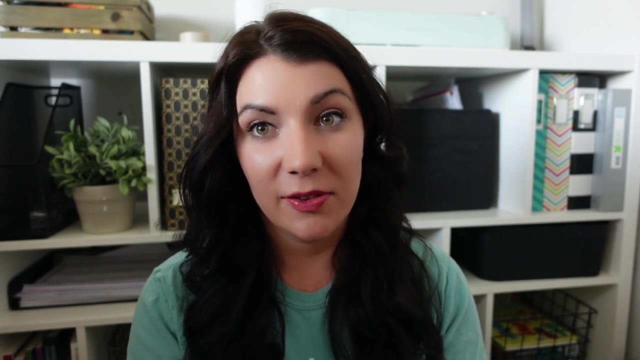 deciphering between that. So that will will be my fifth graders. handwriting, And then moving on to the fun part, is kind of like our reading, what books we're going to be reading, literature guides, unit studies. So we love unit studies, We do a lot of them together and a lot of them end up being 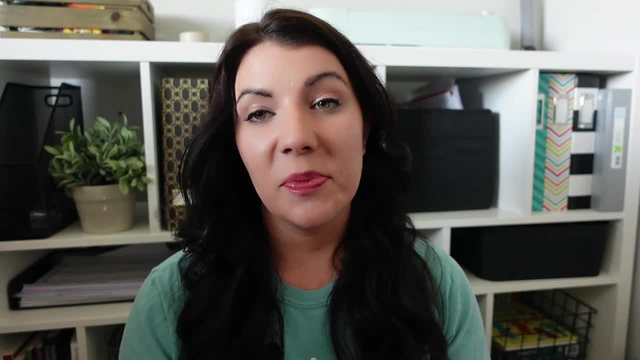 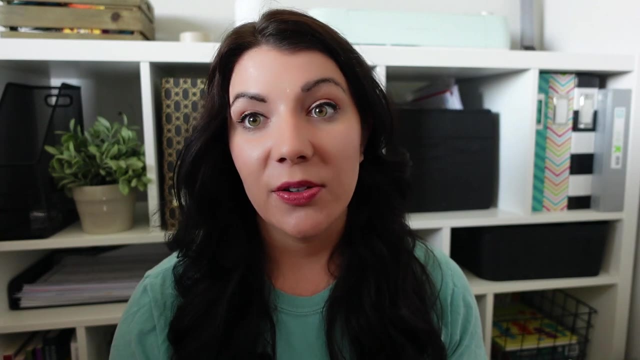 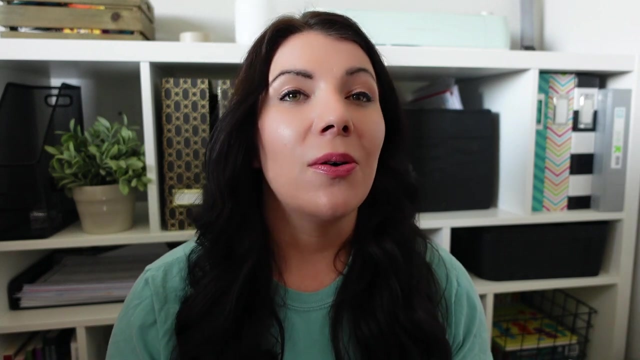 based on reading a book, some language arts in there, So we've been doing a lot of zoom and we've been reading and some reading class. so it's really a great way to help people and then also for our kids to like learn how to read better. we also have like a 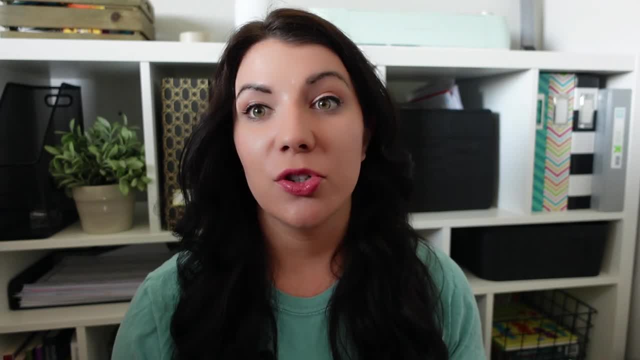 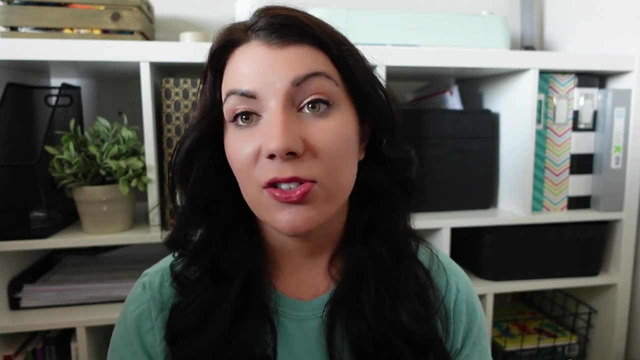 um, so I- just because I feel like we skip through so much of that- I have been on the look for other literature guides. like I said, I really like that. it tells us, like, what lessons to read, what chapters. that just takes something out of my brain. less that I have to schedule and I really like the. 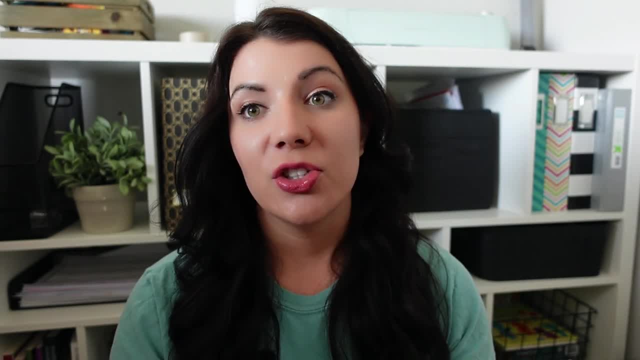 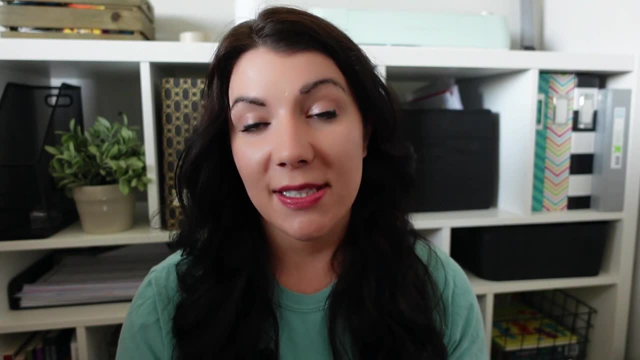 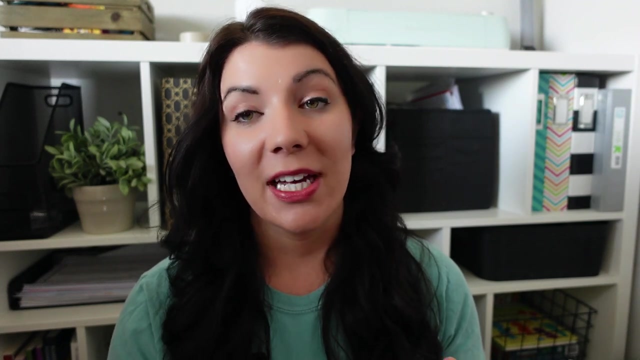 discussion questions with answers, because I work full-time and so normally when they're doing their read-alouds I'm not with them. sometimes I am, but not always because I'm working. so those discussion questions and answers really helps me um one understand what book they're reading. if I haven't. 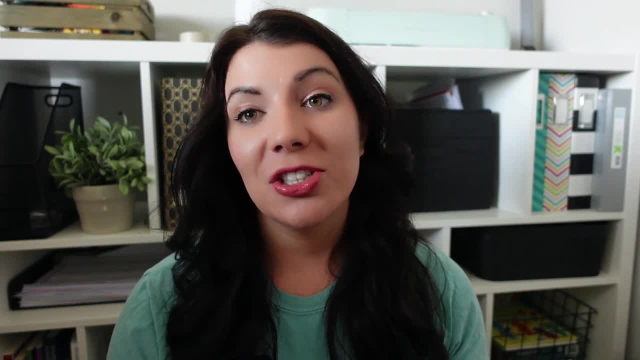 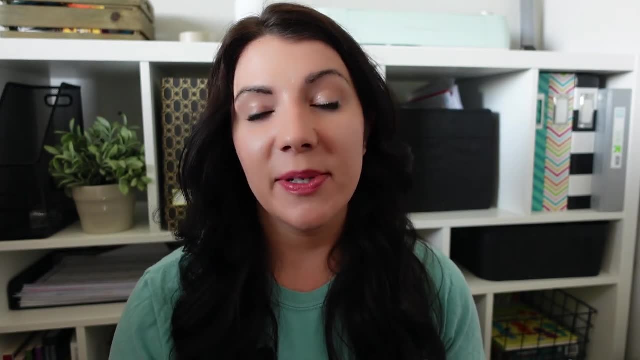 read it already. and two, really make sure that they're paying attention because that they know these questions are coming. so those are really my only requirements in a literature guide is I want it to be cost effective, because we run through them really quickly, um, so they need to be cost. 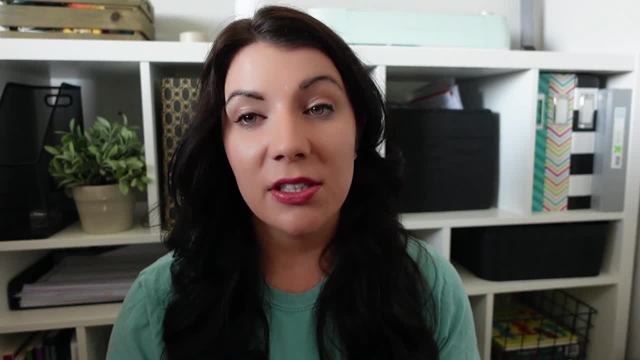 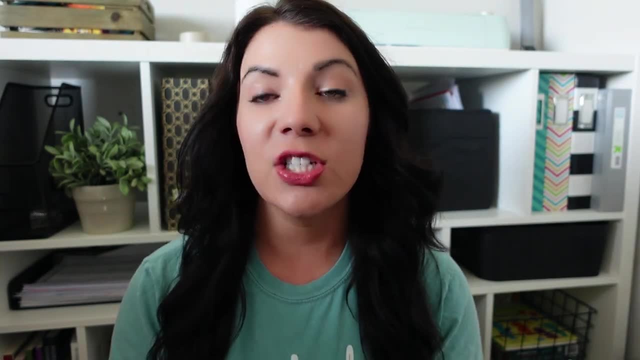 effective and I want discussion, questions with answers and I would like some sort of like: hey, read this chapter, or read these chapters together. so those are my only. requirements are really like my only wish list. so what I'm doing is I went through our homeschool room and 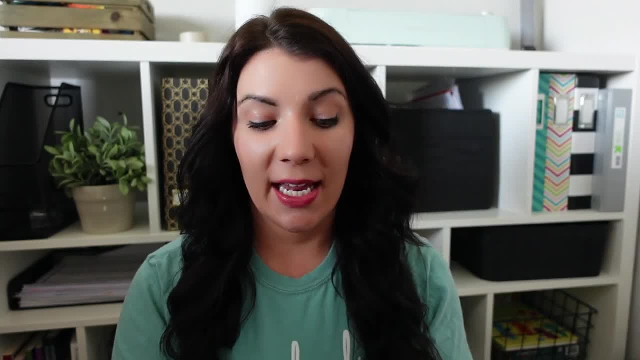 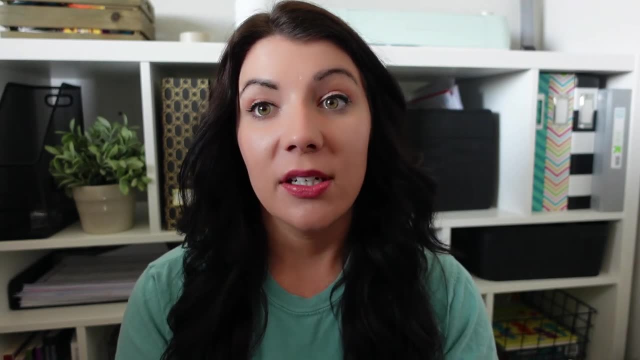 our library because we have so many books and I was like I'm not buying any new books because we have a ton that we need to read. so I had both my daughters pick a book that they want to read this school year and then I picked the rest. um, so I picked all the books first and then I just went. 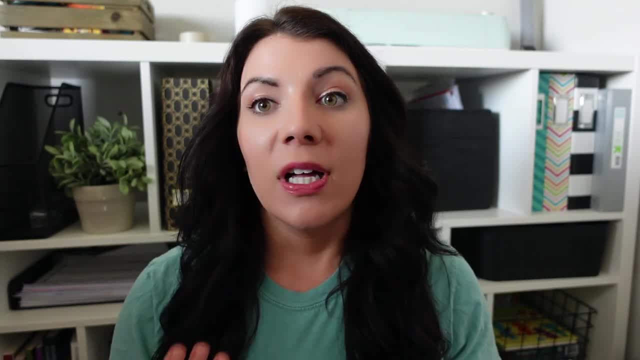 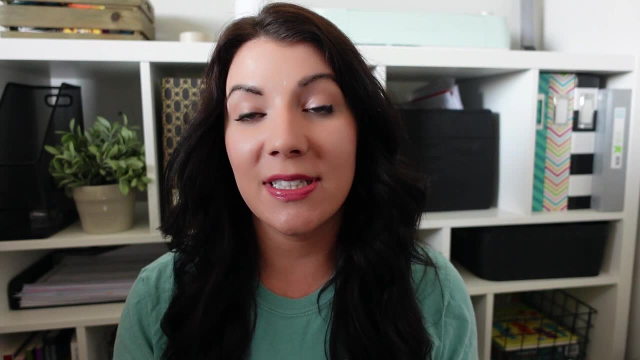 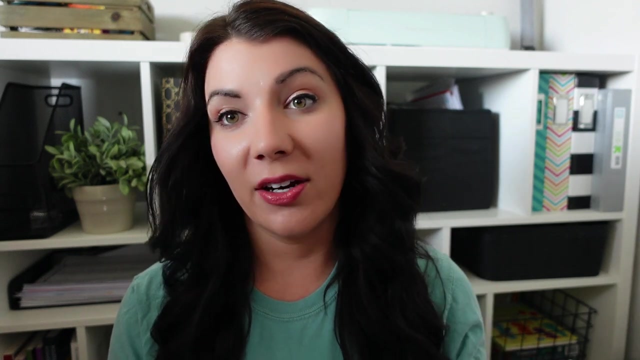 online and started researching. okay, you know this is the book, what literature guides are available and do these literature guides meet my wish list? and so I picked seven books, uh, for the upcoming school year. now I feel pretty confident we'll be able to do that, because we're doing it together. 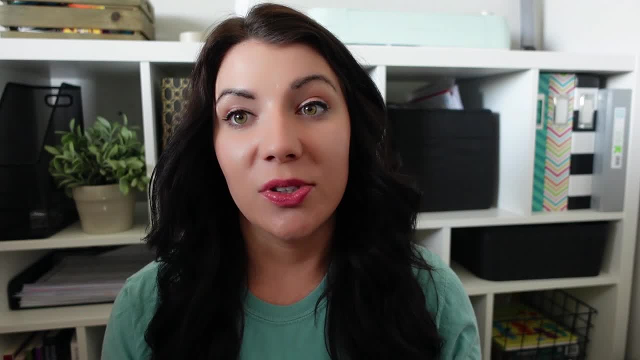 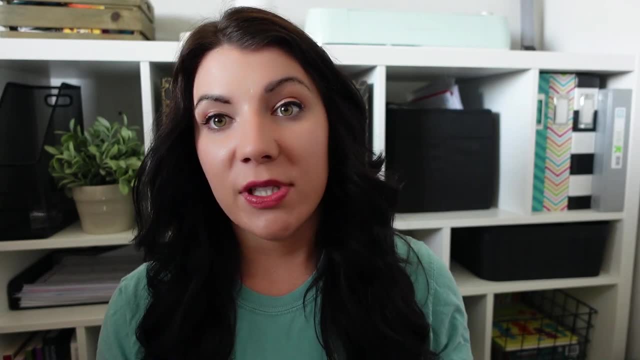 uh, so we already have like a time slot in our homeschool day where we know that reading is happening, and so I feel super confident we'll get through these seven books. there may be more, we'll see. I know I want to do like a Christmas themed one or maybe a Thanksgiving one, but these 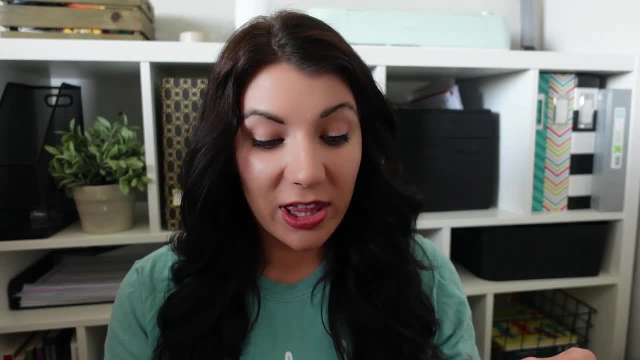 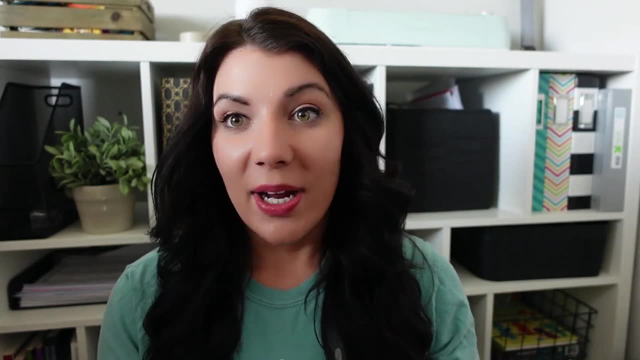 are ones that we'll just work on throughout the year, and so with that, I will have- actually there's eight books- I'm lying, there's eight books, um, and that means there's going to be eight different literature guides, which sounds crazy. right, there's so many literature guides out there that really it's hard to pick, but they're all. 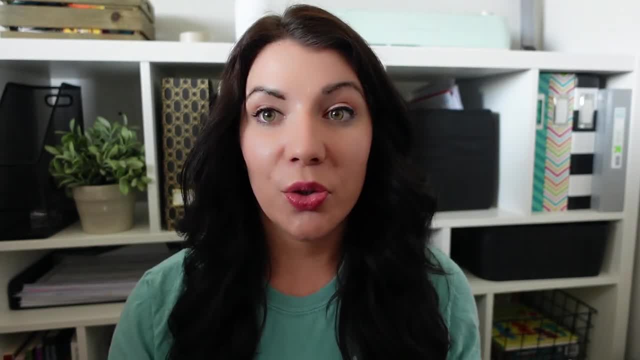 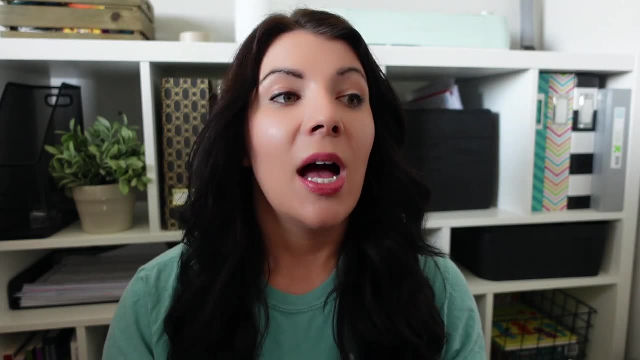 so different at the same time. so I'm going to share the actual books in this video and then, once I actually physically get all the literature guides- because I had to order them all- I'm going to do a separate video on all the literature guides and then I'll do individual videos on each. 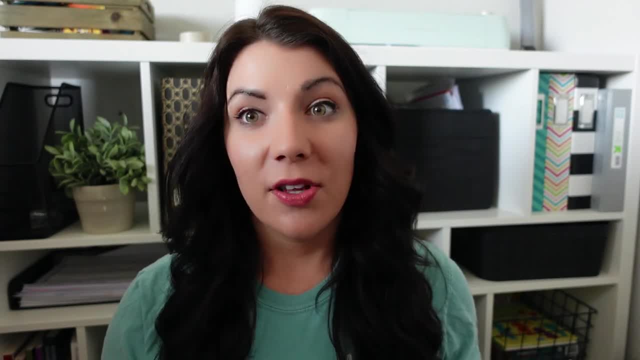 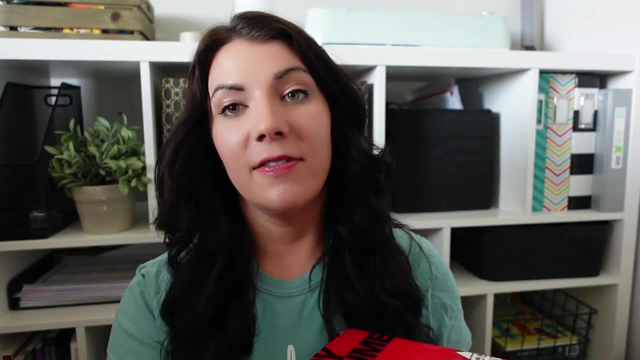 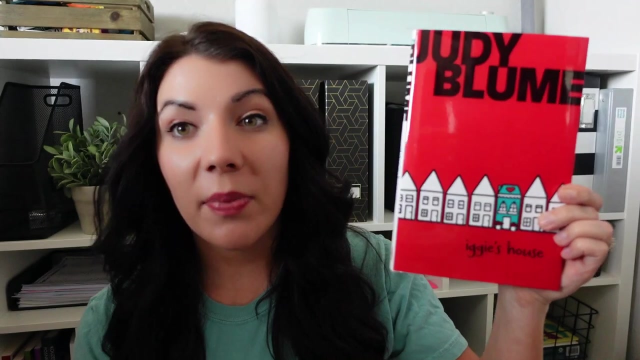 like guide and book together. so lots of those coming out, but that will be way more into the homeschool year, all right. so this is our book stack of the eight books that we're going to be reading over the upcoming homeschool year. we are going to be reading Iggy's House by Judy Bloom. 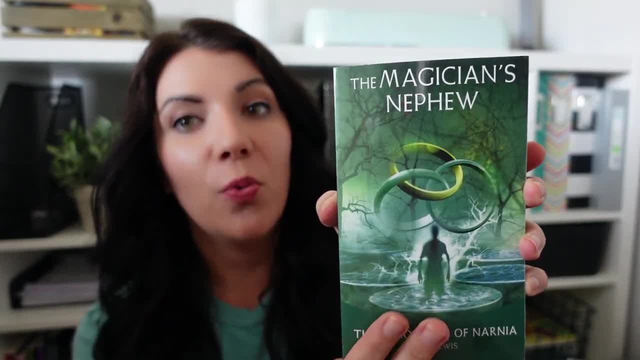 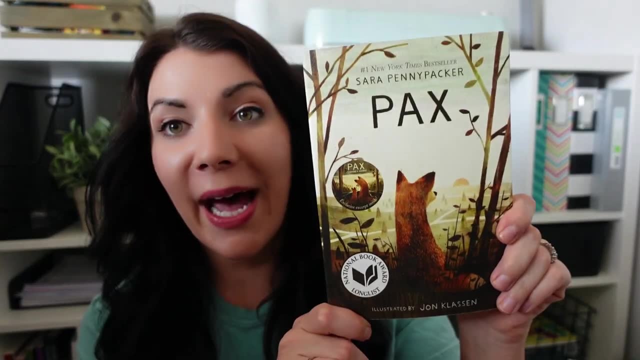 from CS Lewis: The Magician's Nephew- this is book one in the Chronicles of Narnia. and The Lion, The Witch and the Wardrobe, which is book two, Matilda Pax: Bridge to Terabithia. and then these are the two that my daughters picked. so, like I said, I told them 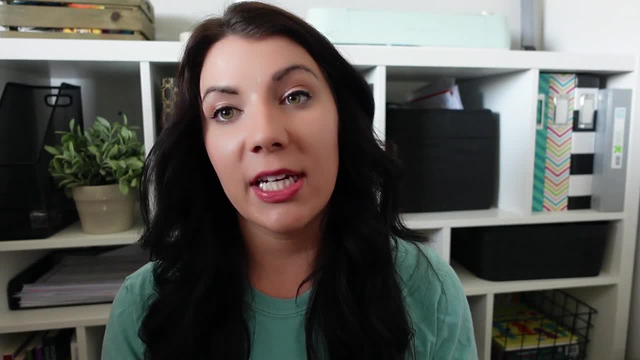 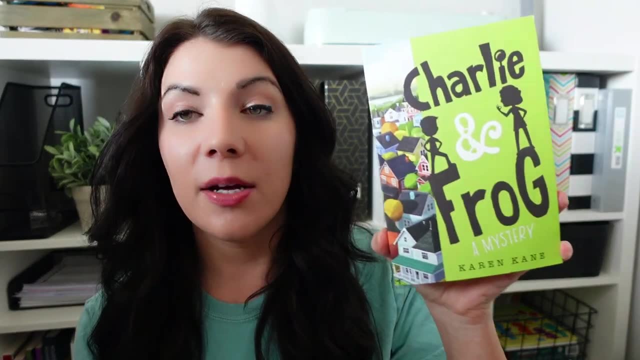 on our bookshelves. you each pick a book. now we're all going to be reading it together, but at least they had a little bit of buy-in of picking it themselves. so my oldest daughter picked Charlie and Frog- a Mystery. we've had this book sitting on our shelves for a while and she's really wanted. 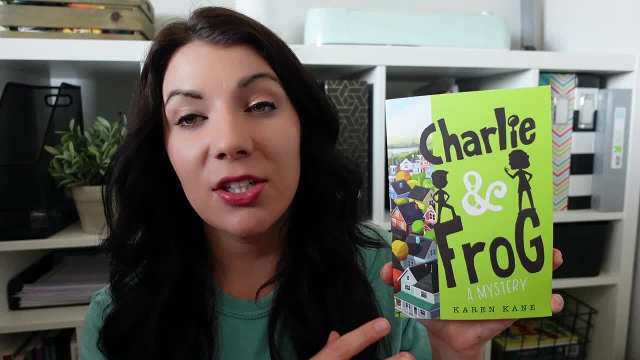 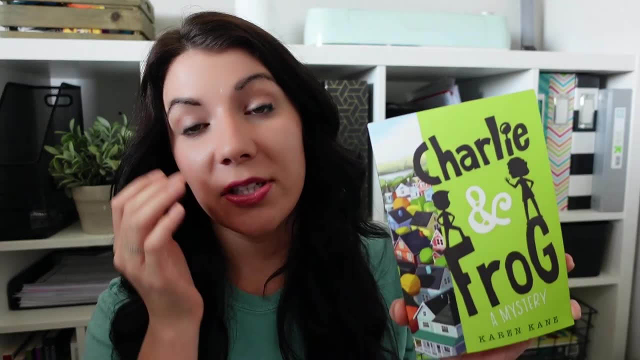 to read it because American Sign Language is incorporated into it and that's the foreign language that she learns and really loves, and so, um, she's really been wanting to read it, so I found a literature guide on it, so we are going to tackle this this year, and then my other daughter, 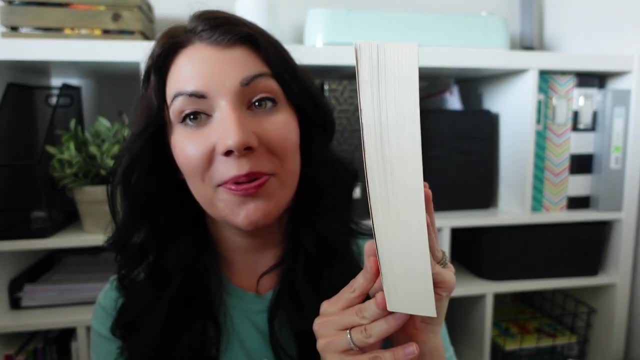 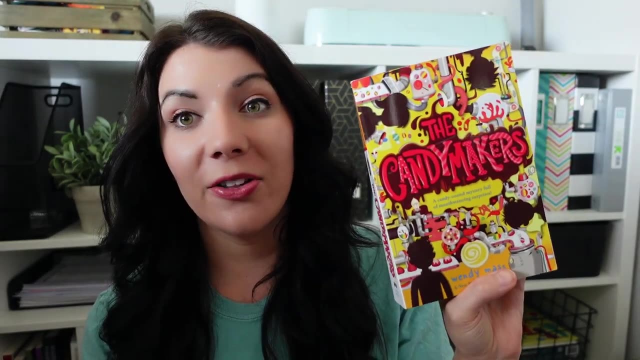 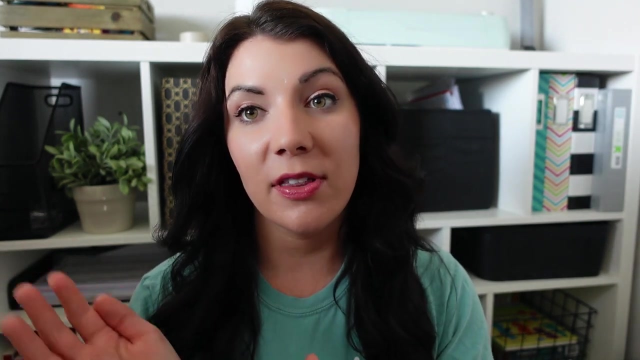 picked the Candy Makers, and so this is a pretty large book. um, I heard it's really good and again, I found a lit guide on it, so we're going to tackle this one as well. so those are. that is everything that my kids- my older two, so my fifth and third grader- are going to be using for language arts, if 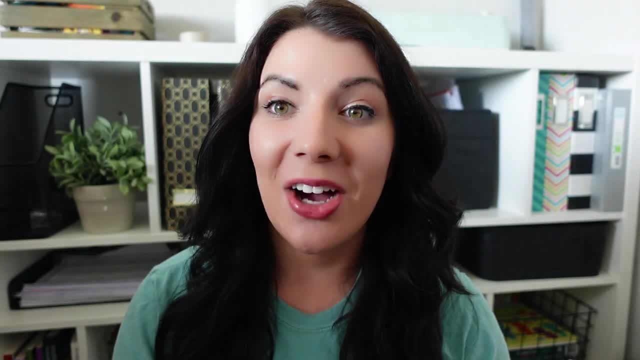 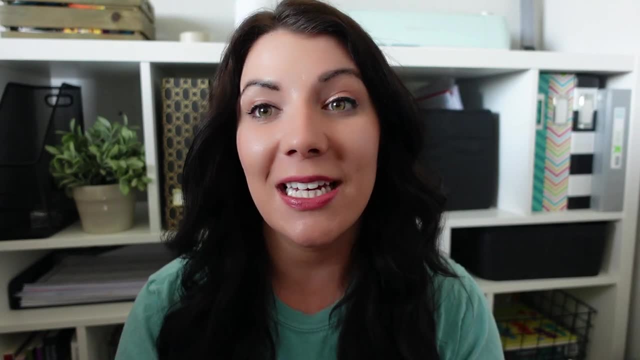 you have any questions, leave those down below in the comments. I always love to read them, so I'm just always love chatting with you guys. I learned so much from your guys's recommendations, so feel free to drop anything down below. also, don't forget that this is a collaboration. Shauna and Devine always.